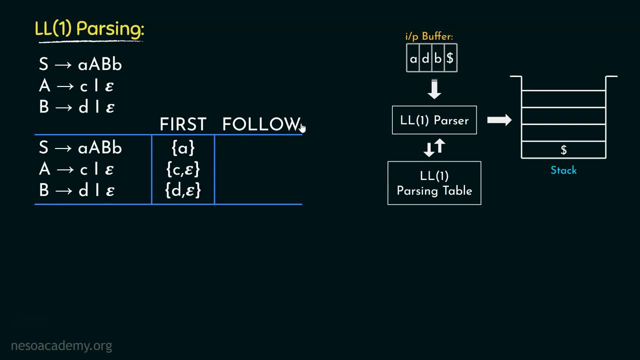 involved in this grammar. Let's begin with the follow now. Now observe carefully: the non terminal symbol S doesn't really appear in any of the right hand side of any of the production rules. Therefore, the start symbol is only going to have the dollar symbol in the follow set. Now, what about A? As you can. 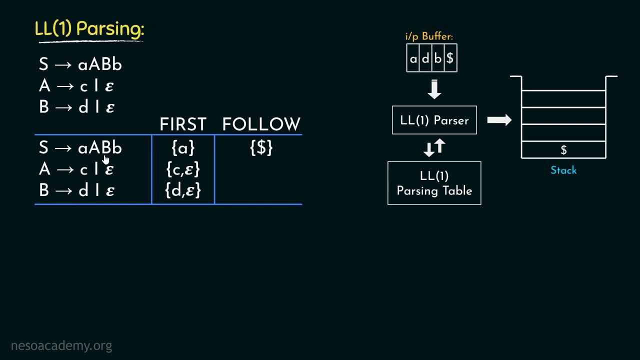 observe: A is being followed by the non terminal symbol, capital B, and the first of B includes the terminal symbol D and epsilon. So definitely for the follow of A it is going to include the terminal symbol D. Now B can also generate epsilon. So in case B generates epsilon, in that case 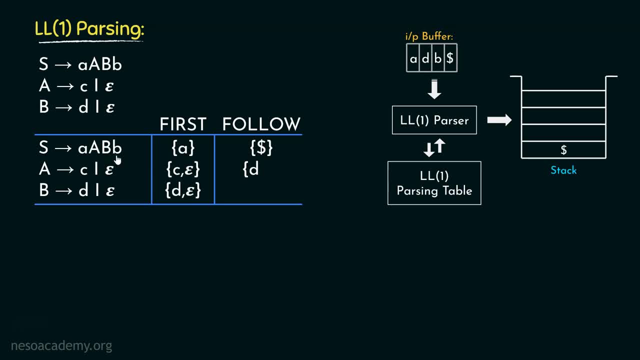 the non terminal A will be followed by the terminal symbol B. Therefore, in the follow of A, alongside the terminal symbol D, we are also going to have the terminal B. Now what about the non terminal B? As you can see, the non terminal capital B is being followed by the terminal symbol small b. Therefore, in 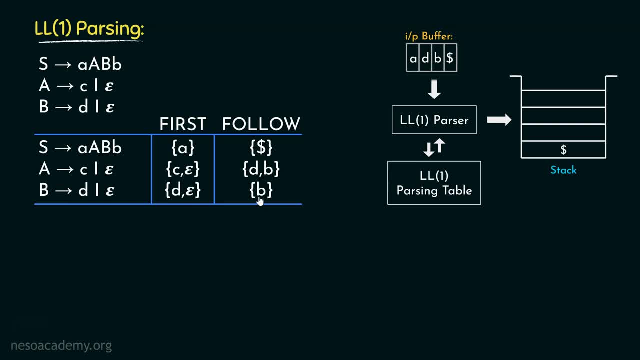 the follow of B. we are going to have only the terminal symbol, small b. So these are all the first and follows of the all the non terminal symbols involved in this particular grammar. Let's now construct the LL1 parsing table. So these are all the non terminals: S, A and B. Let's now find out the terminals. 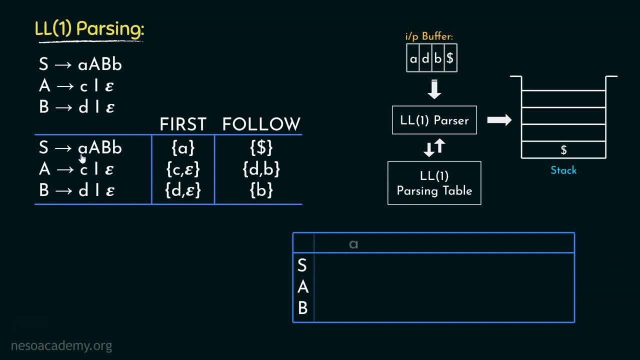 involved in this grammar. So the terminal symbols are A, B, C, D and alongside all these we are also going to include the symbol dollar as a terminal symbol. So let's begin terminal symbol S Now. in the first of S we have the terminal symbol A. So the production. 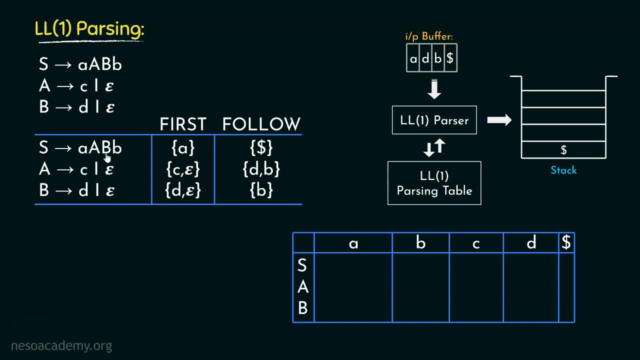 rule S can be rewritten as small a followed by capital A, capital B followed by small c. We are going to enlist this particular production rule in the column of A Now, since S doesn't really produce epsilon. therefore, we don't really need to worry about the follow set. 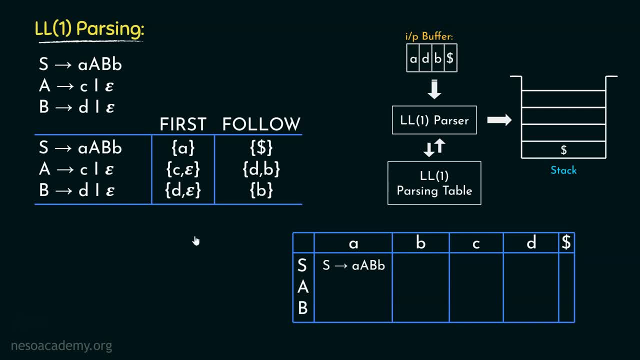 Let's proceed to the next one, that is A. Now in the first of A we have got the terminal symbol c, So the production rule A can be rewritten, as c is going to be placed in the column of c for the row A. Now A has got another production rule. A can be rewritten. 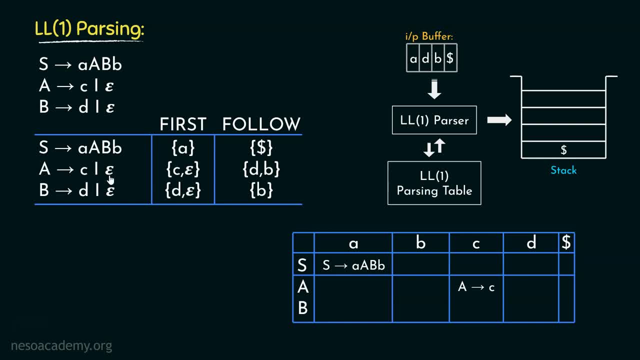 as epsilon. So, basically, A can generate epsilon And since it can generate epsilon, therefore, we need to consider the follow sets And according to that rule we are going to place the production rule, A can be rewritten as epsilon in the columns of D and B. Now let's move on to 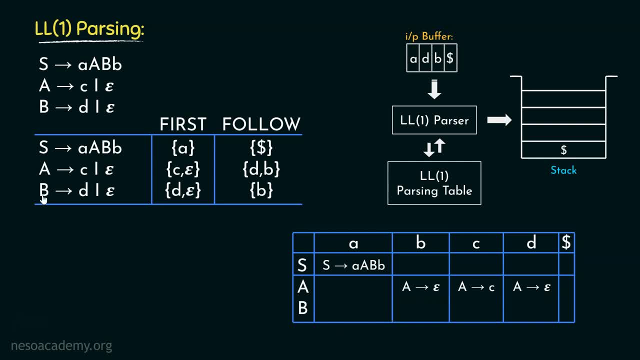 the next non-terminal, That is capital D and B. Now let's move on to the next non-terminal, that is capital capital B. Now, in the first of B, we have the terminal symbol D. Therefore, the production rule B can be rewritten as small. d is going to be placed in the column of D of the row. 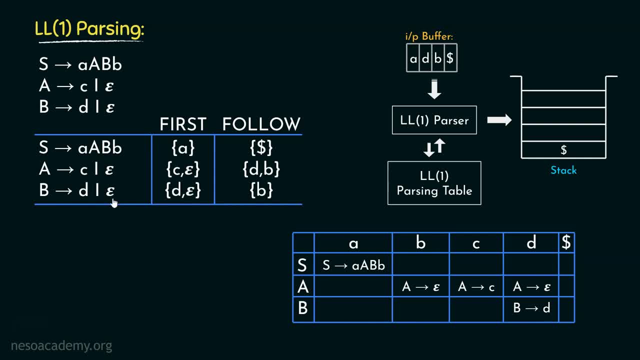 B. Now B can also generate epsilon. Therefore we need to consider the Apollo set. So the production rule B can be rewritten, as epsilon is going to be placed in the column of B. So now we have our entire L1 parsing table. Let's now observe how the parse tree will. 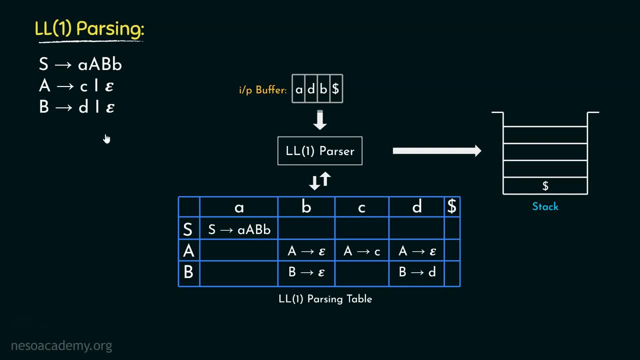 be generated for this particular input string. Now the parsing will begin from the start symbol, which in this case is this S. So we are going to push this particular non-terminal into the stack first. Now observe: S is actually being followed by the dollar symbol in this. 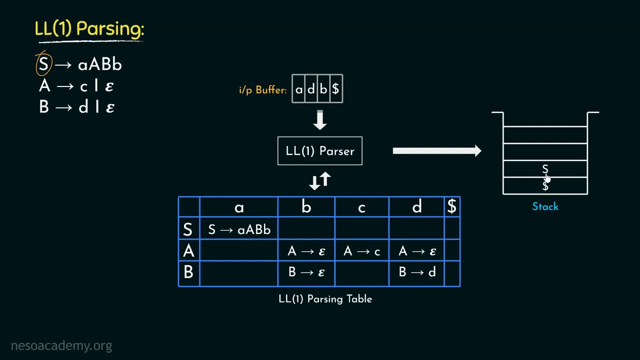 stack And this is the reason why the follow set for the start symbol always includes the dollar symbol. Anyway, let's proceed with the parsing. As you can observe, in the top of the stack we have the non-terminal S And in the input buffer the loop is going. 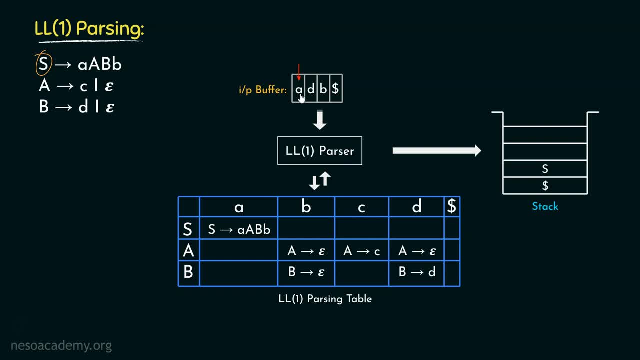 to look at says we have got the terminal A. Now, looking at the L1 parsing table, observe S on seeing A is going to use this particular production rule. So basically, we are going to pop this S. that is this non-terminal, And whenever we pop something, it specifies: 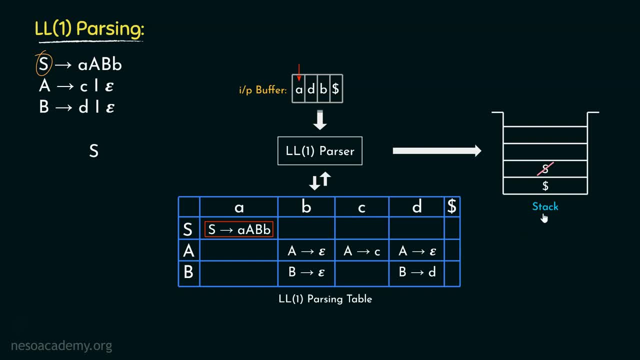 that the parse tree is being constructed Now in the stack. after we pop S, we are going to replace it with the right hand side of the production rule, that is, this particular sentential form. Now, the right hand side of the production rule is going to be stored into the stack in. 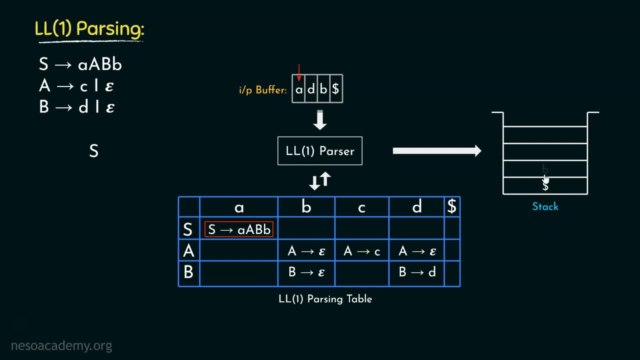 the reverse order, That is, we are going to store small b, then capital B, then A, then small a. Observe, we are maintaining the order. Now. this basically means from S: we are trying to derive this particular tree, But we are yet to derive it. This is just the structure. 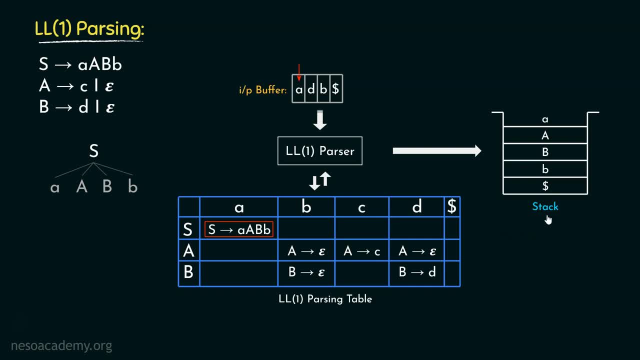 that we are going to derive. Now focus on the stack. In the top of stack we have the terminal symbol A. In the input buffer we also have the terminal symbol A. So this C is a match And whenever it's a match, we are going to pop the symbol from the stack And by popping it we are 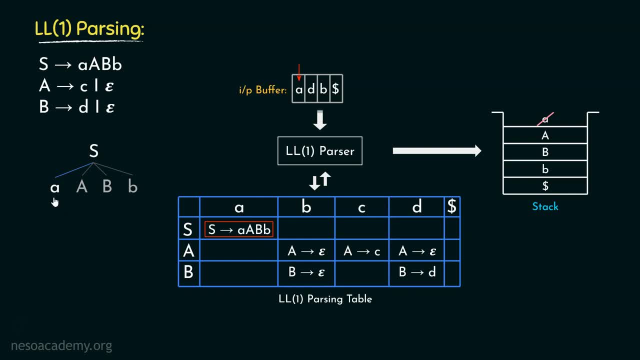 specifying that this particular branch of the tree that S derives. this A is being finalized now. Now, since we have matched one terminal symbol from the stack, popping of it will signify that we increase our input buffer scanning. So now in the input buffer, the lookahead. 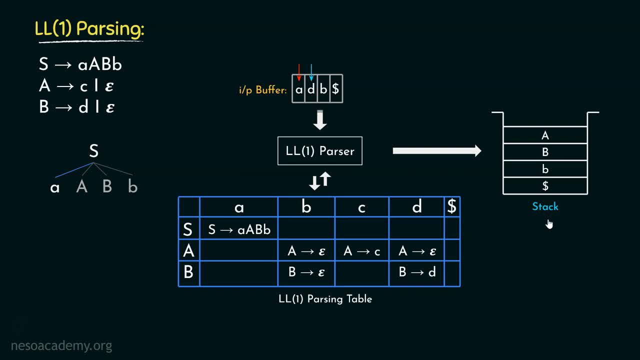 is saying the terminal symbol is small, d. Now notice the stack. On the top of the stack we have the non-terminal capital A. Now for the non-terminal A. if the parser sees the lookahead as d, then from the L1 parsing table. 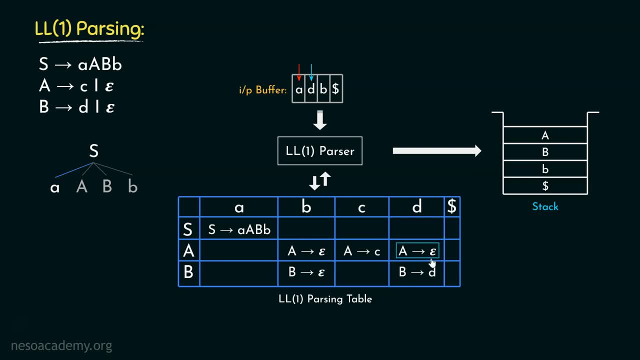 it is going to choose this particular production rule. That is, A can be written as epsilon, So we are going to pop A from here now And popping A will mean that we are finalizing this branch of the tree that is S can derive capital A Now after popping A, due to the 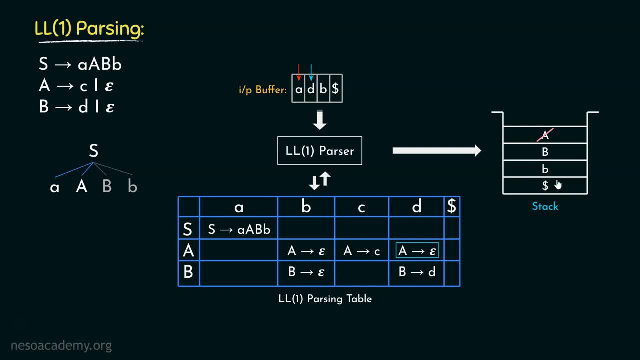 production rule. A can be written as epsilon, and popping A means that S can derive capital epsilon. the top of the stack will be replaced with epsilon. Now, coming to epsilon, it actually means empty string, So we will pop it And this will finalize the derivation: a derives epsilon. 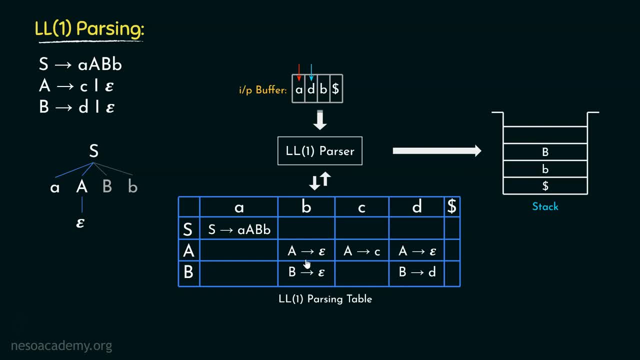 in the parse tree. Now, once epsilon is popped, observe the stack. we have got the non-terminal capital B in the top of the stack. Now in the input buffer we have the terminal symbol D. So, coming to B, seeing the terminal symbol D in the input buffer, the L1 parser is supposed to 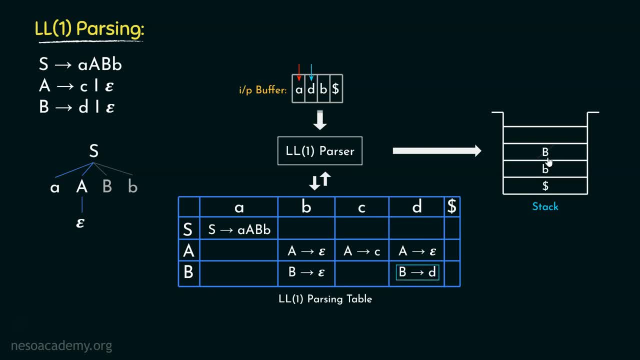 choose this particular production rule. Therefore, B will be popped, And by popping B, we are finalizing that this branch of the tree that s can derive B is getting finalized Now. once B is popped, it will be replaced by the terminal symbol D. now. Now, as you can see in the top of stack. 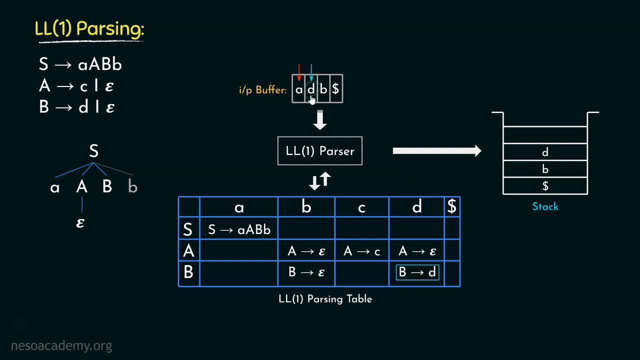 we have D and also in the input buffer we have D. So this is a match. And since it is a match, we are going to pop D, which will finalize the derivation. B can derive D Now, since the terminals in the top of the stack and in the input buffer match. therefore, we are going to 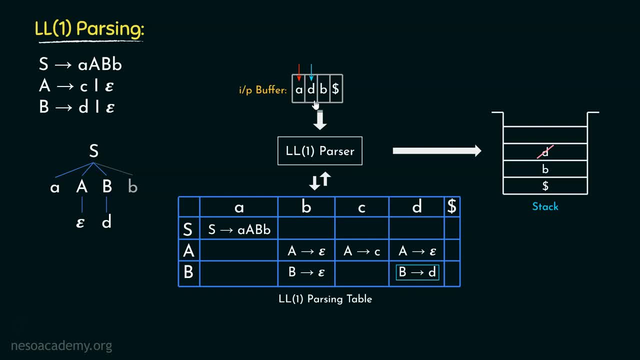 increase the scan That is now in the input buffer. the lookahead will move to the next terminal symbol, that is B. Now observe the top of the stack. it is having the terminal symbol B. So it is basically a match, isn't it? So we are going to pop B, which will specify that this. 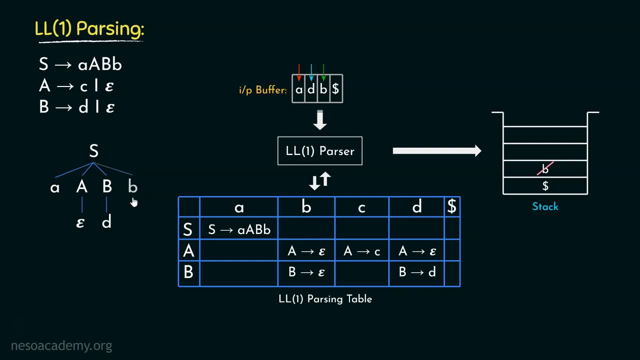 particular branch of s that s can derive small b is finalized. Now, since the terminals match, therefore, we are going to increase the scan that is now in the input buffer. the lookahead will move to the next terminal, symbol B. So now the lookahead will get to the symbol dollar. 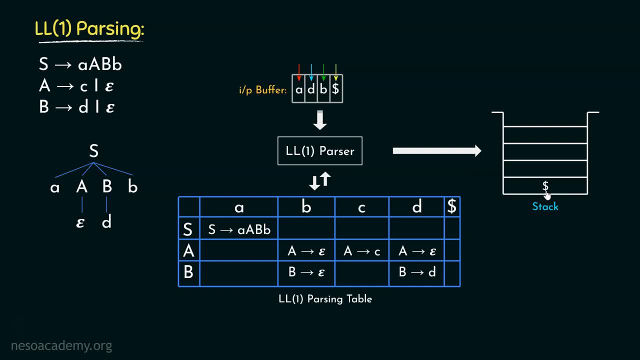 Notice the top of the stack. it is also having dollar. so it is a match, isn't it? Now, in an LL1 parsing, as you have observed, whenever we match any terminals from the input buffer and in the stack, we practically construct the parse tree. And finally, 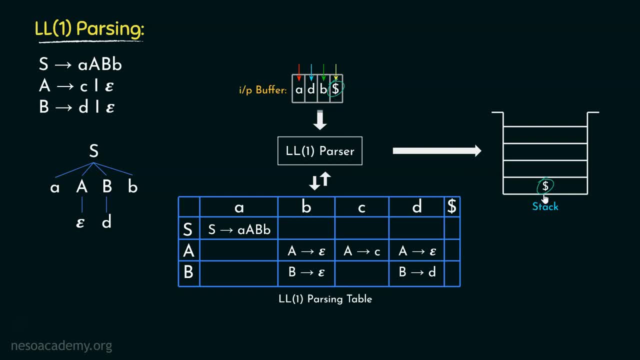 when the input buffer symbol dollar matches the top of the stack dollar, it means the parsing is successful. And if you observe the parse tree, that also yields the same input: A, followed by small d, followed by small b. It was our input right, So this is how the entire 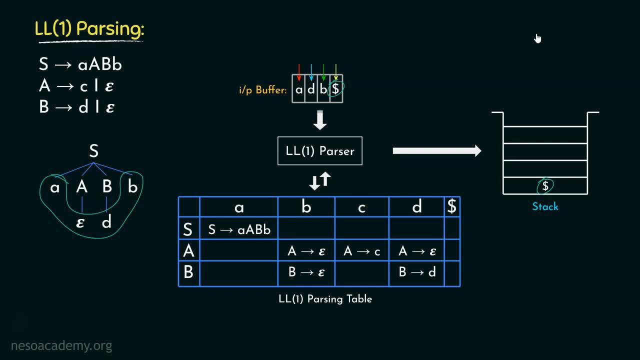 LL1 parsing takes place. Do remember whenever we replace any non-terminal in the stack with its right hand side. in that case all those elements in the right hand side will be pushed in the stack in reverse order, And also the lookahead in the input buffer. 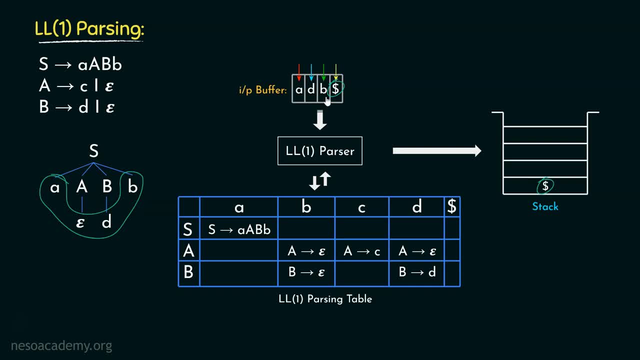 will only move forward whenever we match a particular terminal. And finally, when the symbol in the input buffer, dollar, matches the dollar symbol in the stack, that will signify the successful parsing. And one more thing to remember: the grammars which are good for LL1 parsing are also known as LL1 grammars. Now we 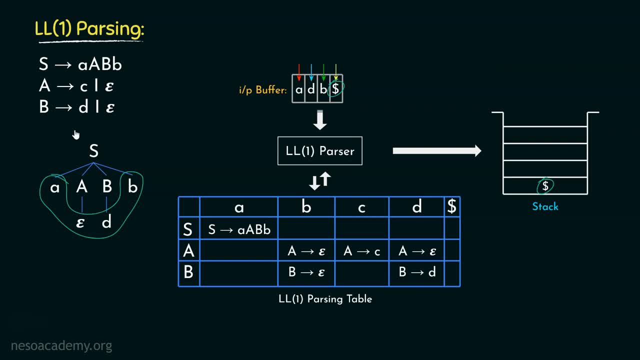 can find out whether a context-free grammar is LL1 grammar or not once we construct the LL1 parsing table for that particular grammar. Now, how is so Observe for every non-terminal considering a terminal symbol, we only have a single production rule, isn't it? As you can see, it's the same case for all. 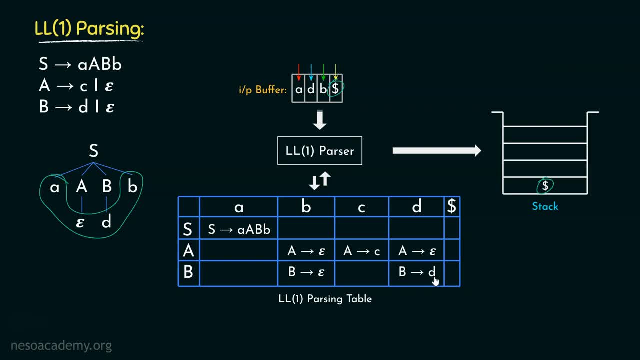 the non-terminals. So if for a particular terminal there exists more than one production rule involving a non-terminal, in that case the predictive parser won't be able to predict what production rule to use, And thus that's particular grammar will not be an LL1 grammar.